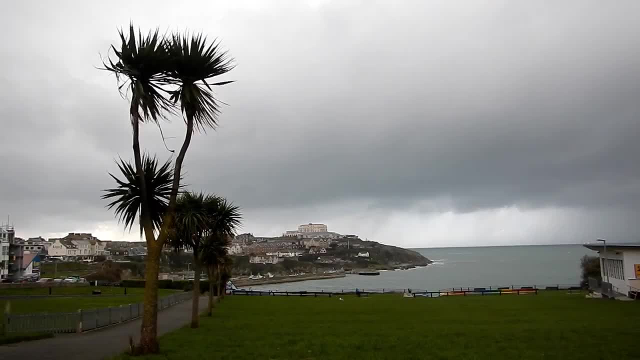 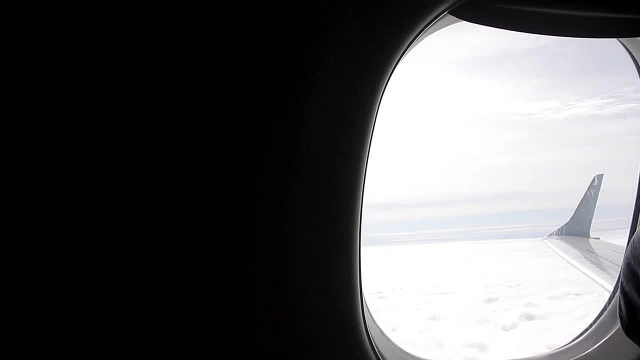 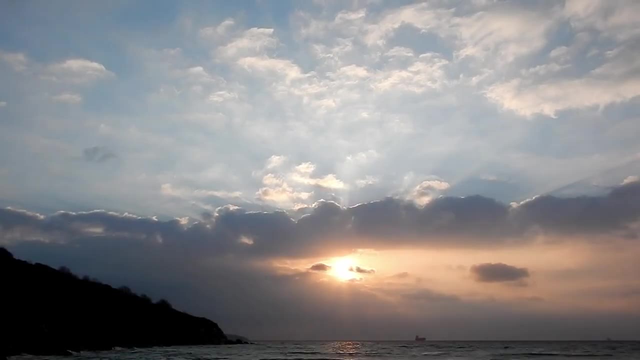 also lower air density. This is because the lighter water vapour molecule will displace a molecule of heavier oxygen or nitrogen. Cold, dry air will therefore be noticeably denser than warm, moist air. The average weight of air in the atmosphere per square inch is 14.7 pounds, which exerts 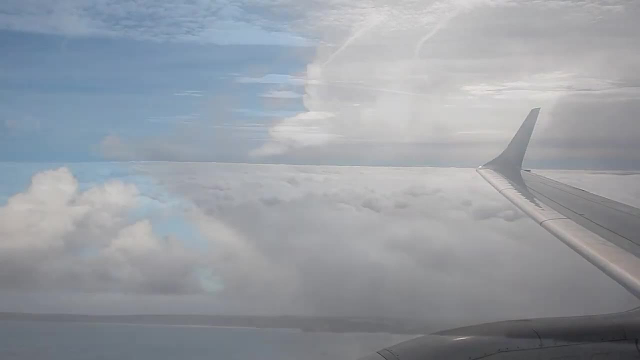 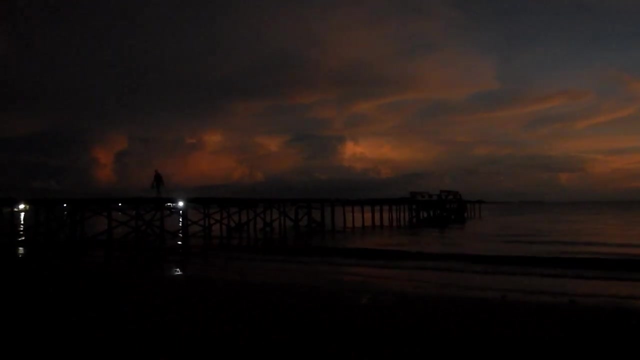 one atmosphere of pressure. Changes in air density will change this standard atmospheric pressure. High and low pressure zones result, which influence weather patterns across the globe. Air will flow from high to low pressure zones around the globe. This is the market in which air will flow. 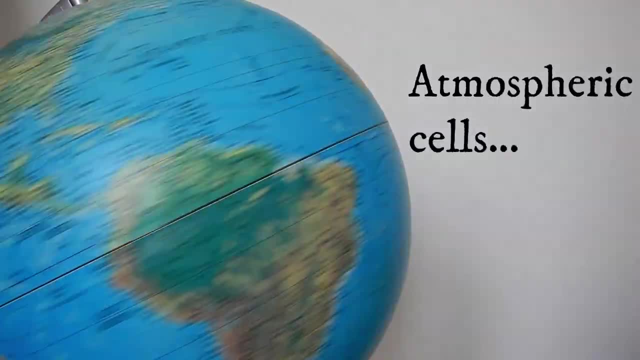 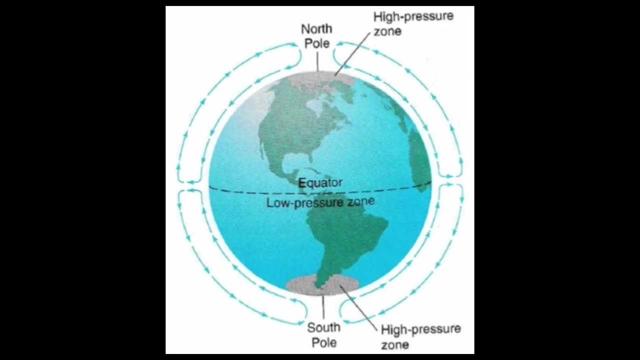 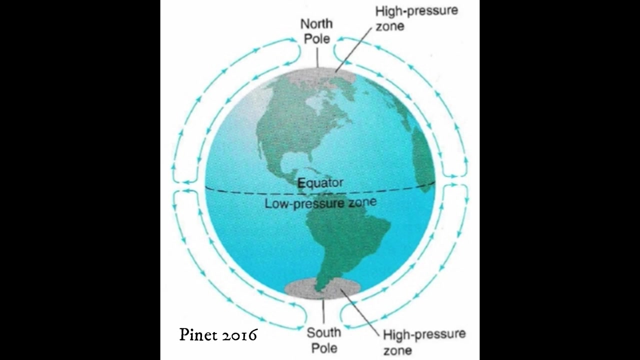 zones creating winds. Imagine the Earth has stopped rotating. Air circulation would be simple between the equator and the poles. The intense solar radiation at the equator would cause a low pressure zone with less dense air rising and diverging. When arriving at the North and South Pole, this air would hit a high. 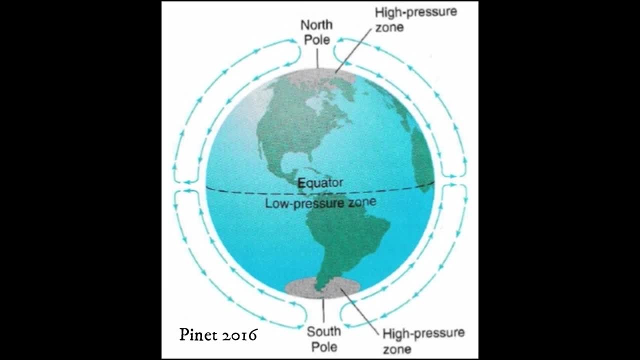 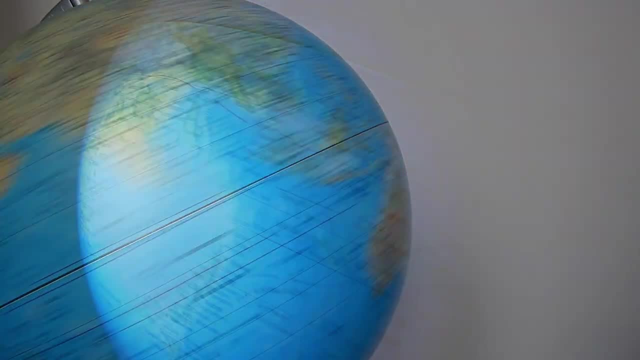 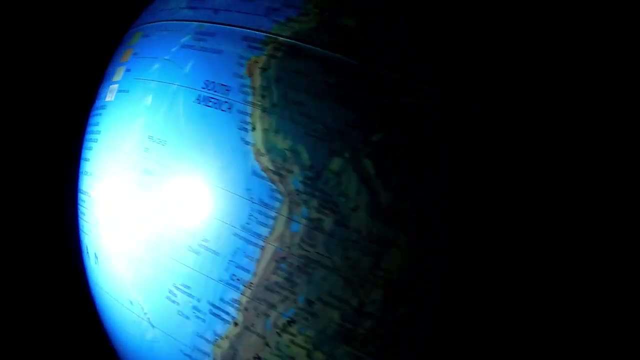 pressure zone of bitterly cold temperatures, The denser air would converge and sink, heading back to the equator for the process to start again. However, the Earth's rotation changes this simple model. Air and water become under the control of the Coriolis effect, where moving objects on a rotating sphere 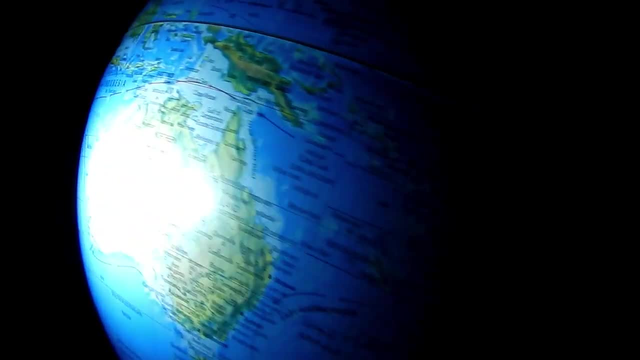 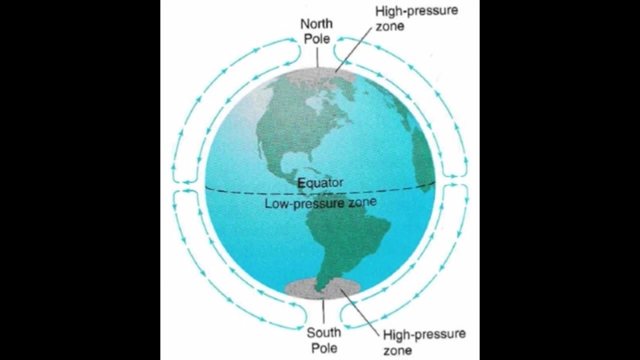 will be deflected. The deflection will be to the right in the Northern Hemisphere and to the left in the Southern Hemisphere. Because of its wider circumference, the speed of rotation will be greater at the equator than at the poles, For example. this doll is travelling faster on the edge of the 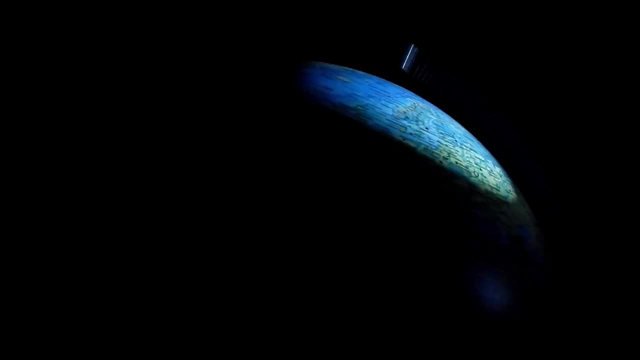 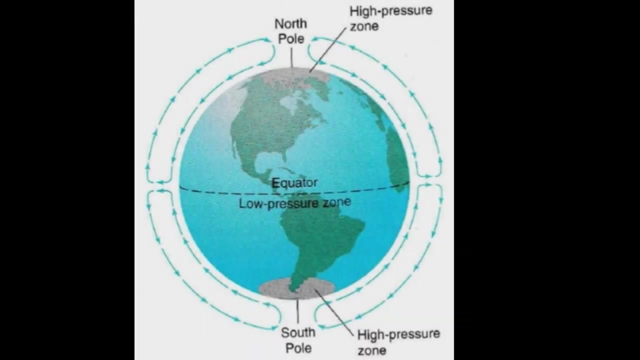 roundabout than the garden frog in the center. The extent of deflection is therefore increased with latitude away from the equator as the difference in speed amplifies. Given these facts, the simple model of air circulation from a non-rotating Earth would change into an increased number of. 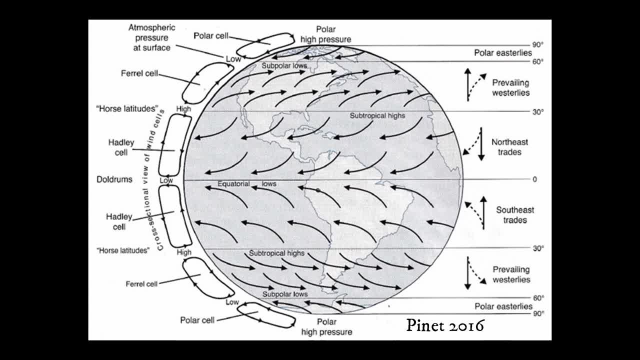 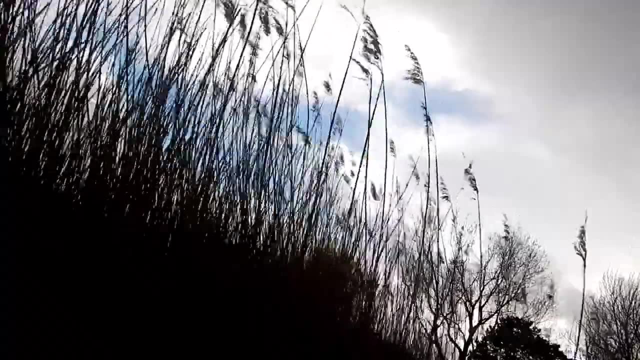 smaller atmospheric cells. Each hemisphere has three theoretical cells: Hadley, Ferrel and Polar. Where the convection cells meet, a band of high or low pressure is created, depending if cool air is sinking or warm air is rising. These theoretical cells create global patterns for wind and air conditions such as the northeast and southeast. 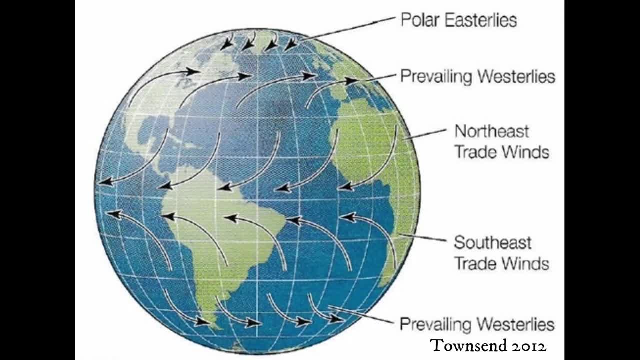 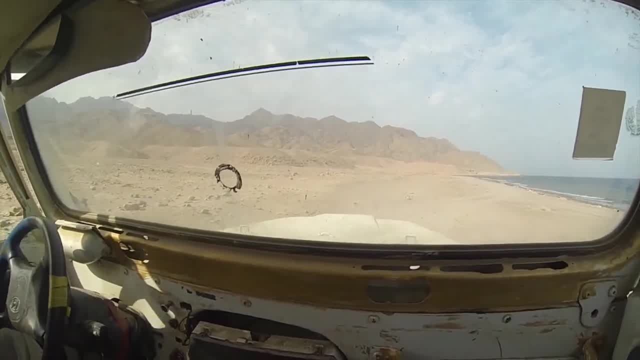 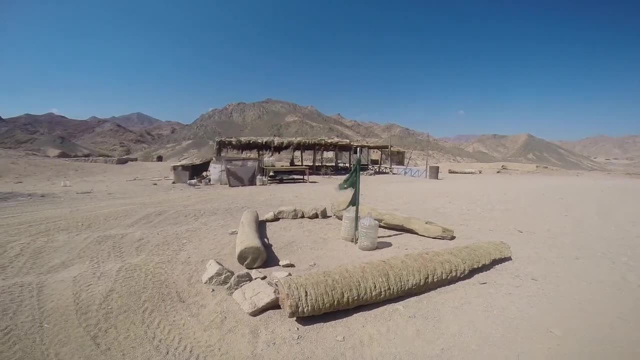 trade winds. either side of the equator prevailing winds and jet streams. High pressure bands would be low in humidity, so areas here typically experience low levels of cloud and rain. Consequently, the planet's major deserts and strips of ocean with weak surface winds can be found at these 30 degree latitudes. The 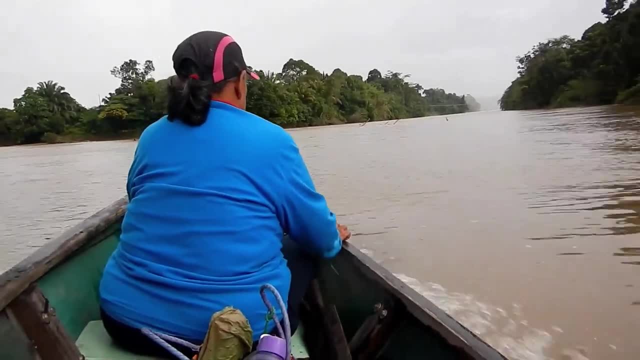 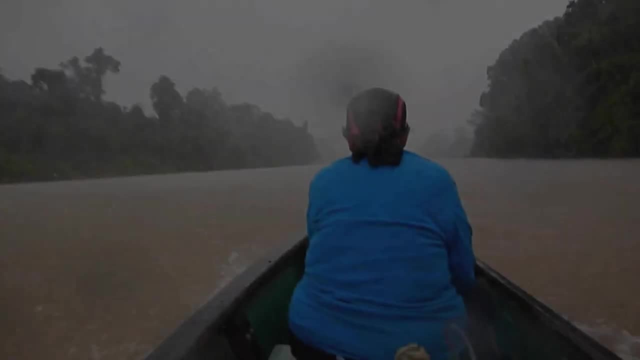 equator is characterized by light, variable wind because most air is rising vertically. The air is also humid, So water vapors condense into small liquid droplets. Clouds and rain result: Momentum from the wind creates surface currents. Like the wind, this surface 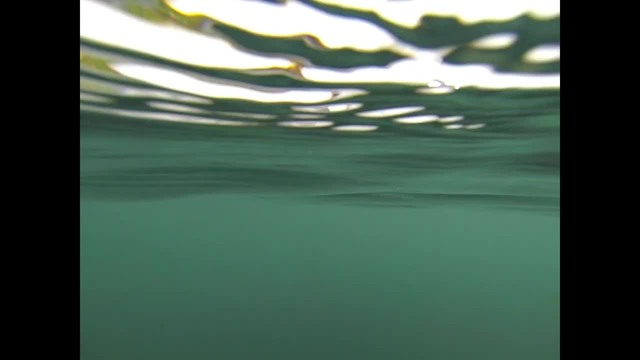 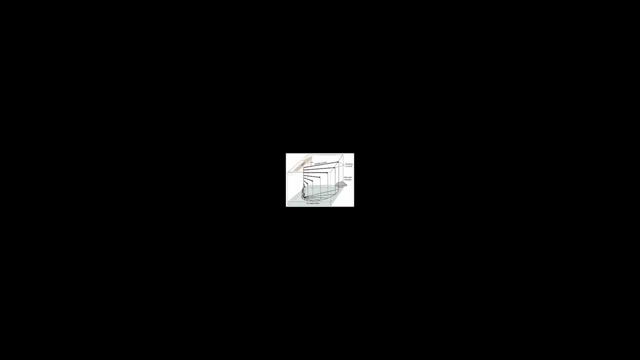 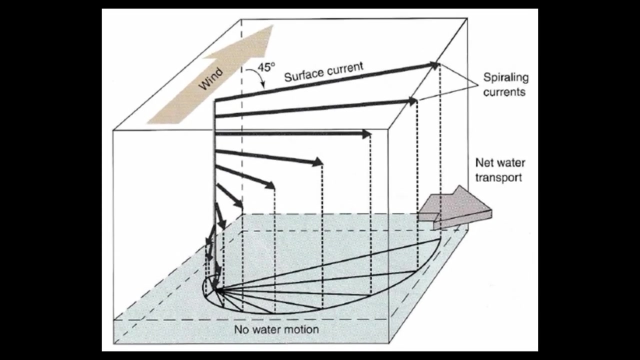 current is manipulated by the Coriolis force on rotating Earth. Instead of the thin layer of surface water flowing directly downwind, it will flow at 45 degrees from the wind direction. This thin surface layer then passes on its momentum through frictional drag to the layer of water below it. although some 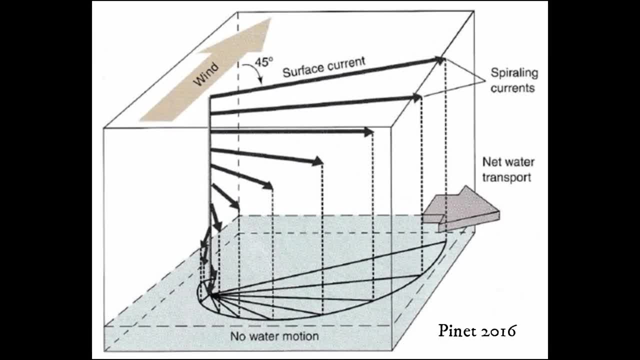 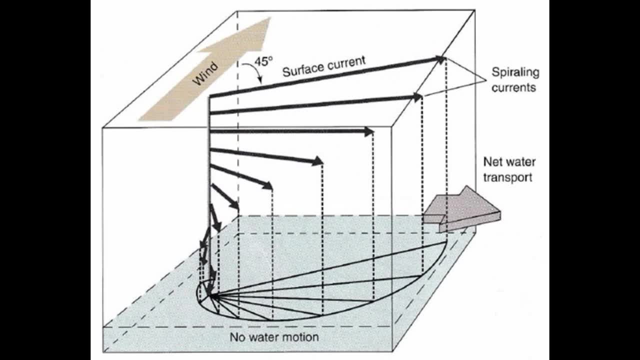 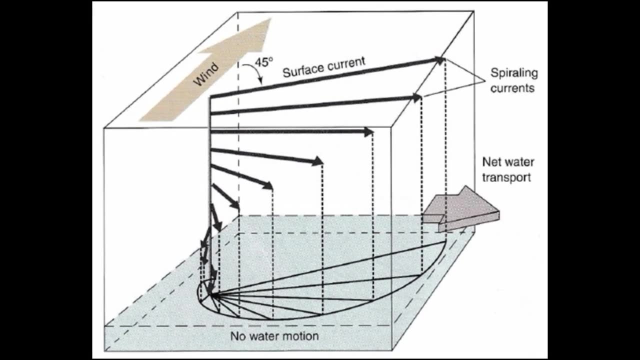 energy and speed is lost. Usually, this second water layer will want to run in the same direction as its neighboring layer, but eventually it too is dictated by the Coriolis effect and deflects further. This process is continued downwards into a twisting current known as the Ekman spiral, which eventually stops at the Ekman depth Here. 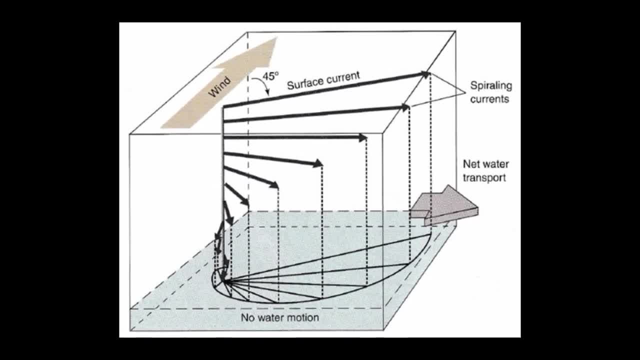 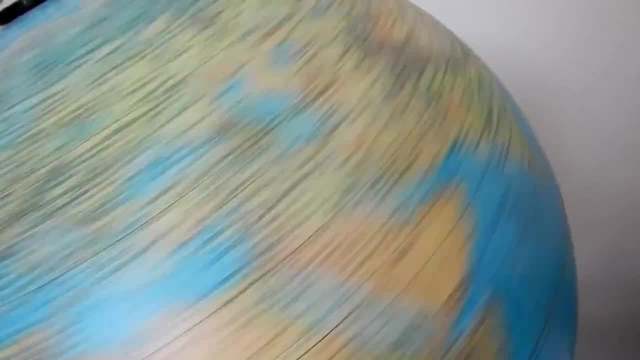 the combined average of the spiralling water above is flowing at exactly 90 degrees from the wind stress. The major ocean gyres are formed because of these currents and wind patterns. For example, in the North Atlantic, prevailing west leaves blow in the opposite direction to the northeast trade winds below it. 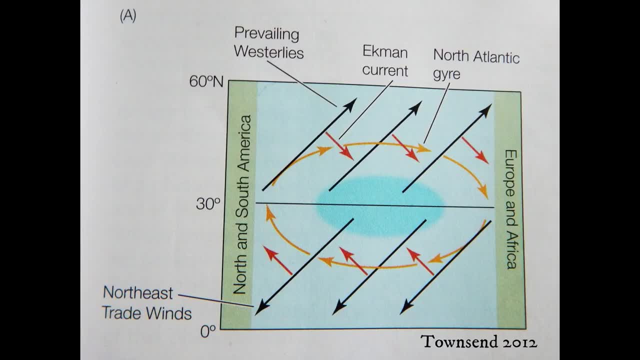 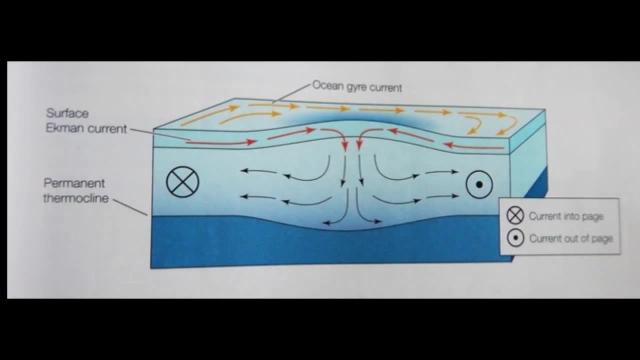 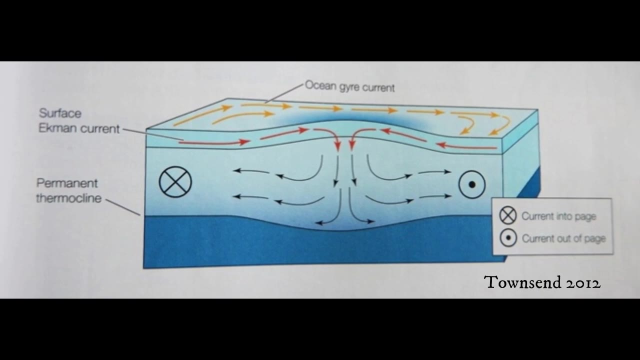 Because the Ekman currents flow at 90 degrees to the wind, surface water is directed into the center of the basin. Water is elevated higher as a result. This hill of water cannot continue to rise, so instead sinks and is only stopped by the permanent thermohaline between 800 to 1000 meters. Once this 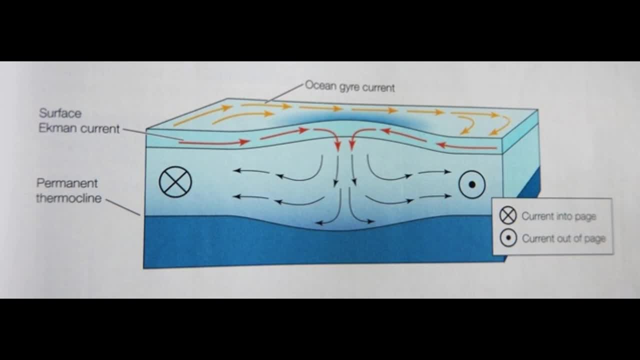 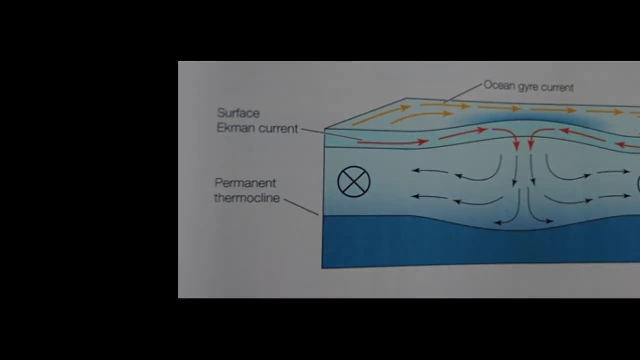 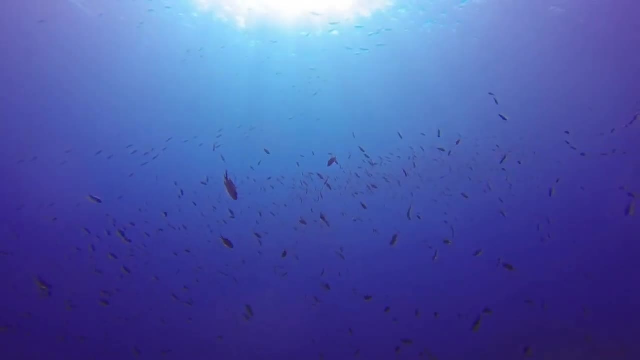 central sinking water has passed the Ekman layer, it begins to spread laterally. However, the Coriolis force commences again to transform the spreading water into a circular gyre flowing clockwise. The elevated sea level created a pressure gradient forcing the water downslope. The currents will eventually be balanced between this force and the 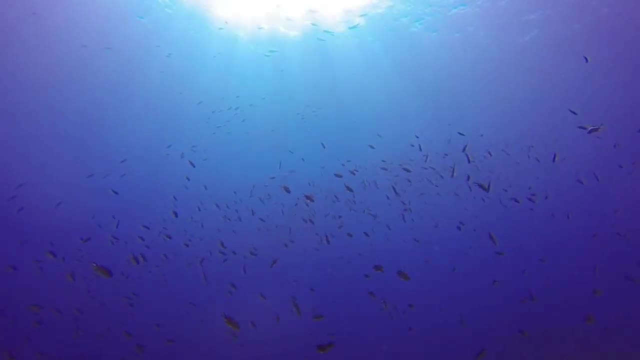 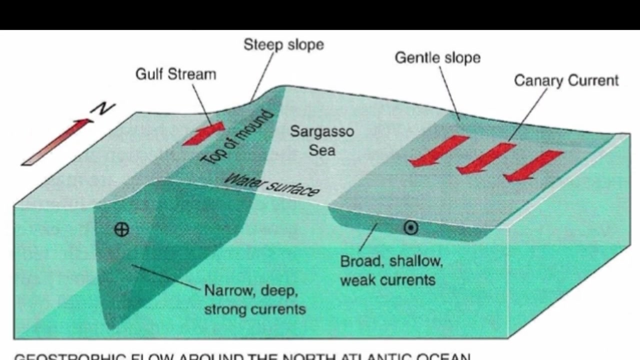 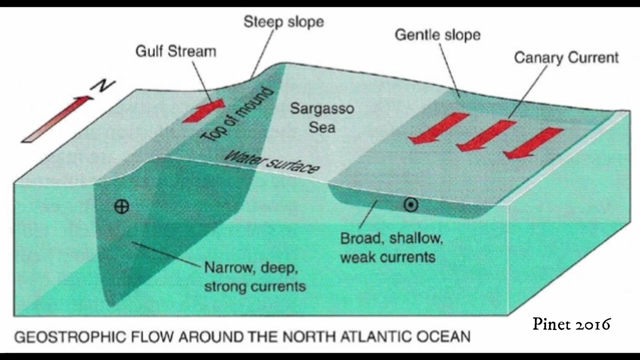 Coriolis force and become known as geostrophic currents. The gyres discussed so far have been theoretical. In the real world, they are asymmetrical and suffer from Western boundary intensification. This means that in all oceans, currents on the western side will be narrower, deeper and stronger than those in the. 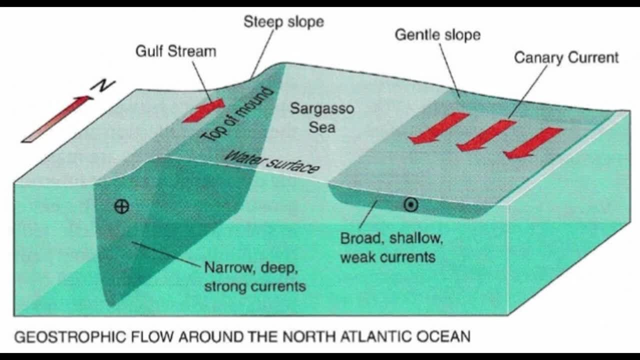 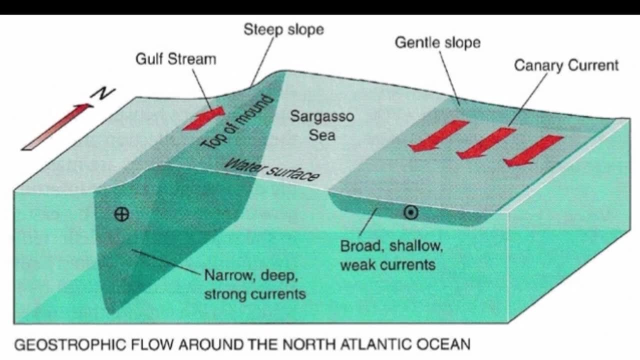 east. The reasoning for this relates back to how the Coriolis effect intensifies from the equator to the poles Within the gyre. the currents are therefore changing direction at different speeds, resulting in contrasting currents and the hill of water being displaced west Examples of these swift 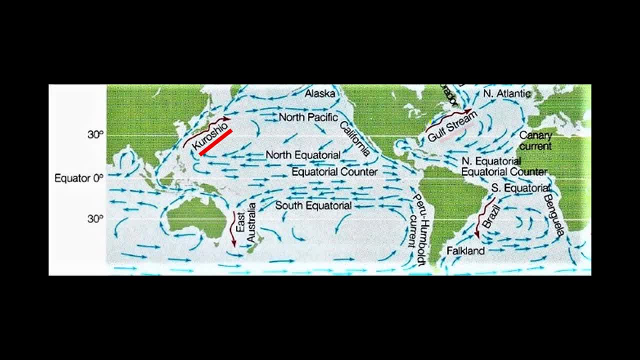 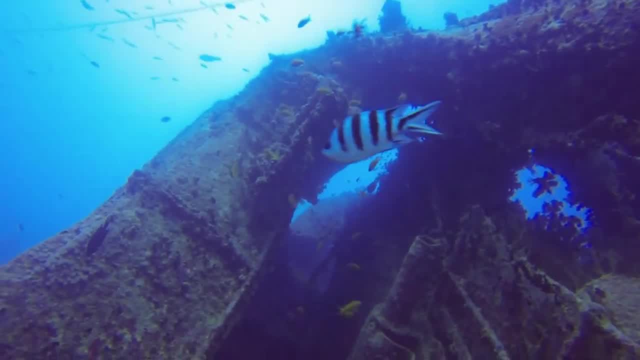 flowing currents are the Corotia extension in the North Pacific and the Gulf Stream in the North Atlantic, both of which on the western edge. But how does water flow in the deep ocean below 1,000 meters? Water currents are density driven through change in salinity and 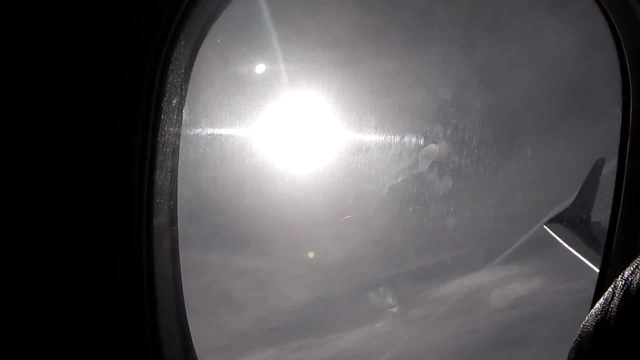 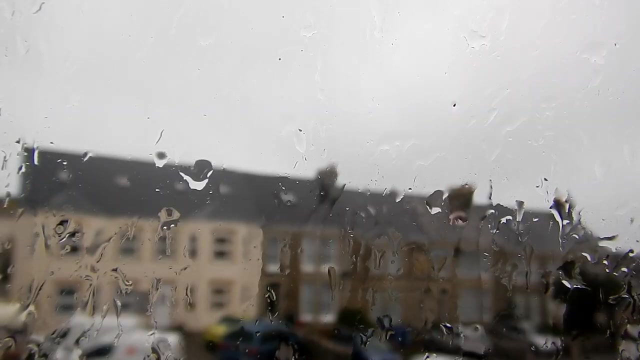 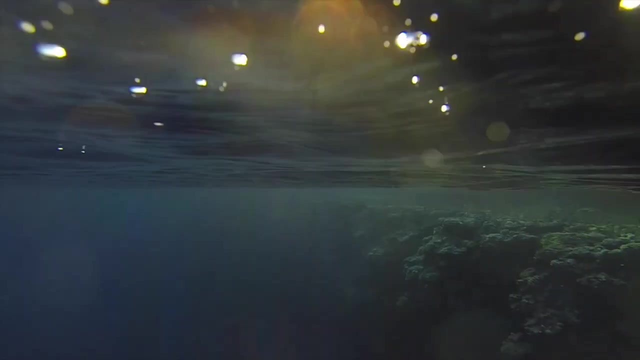 temperature. The Sun is the clear controller of temperature, but also of salinity, due to weather related evaporation and precipitation. An increase in salinity will increase the water's density. In comparison, an increase in temperature will decrease the water's density. A denser body of water will 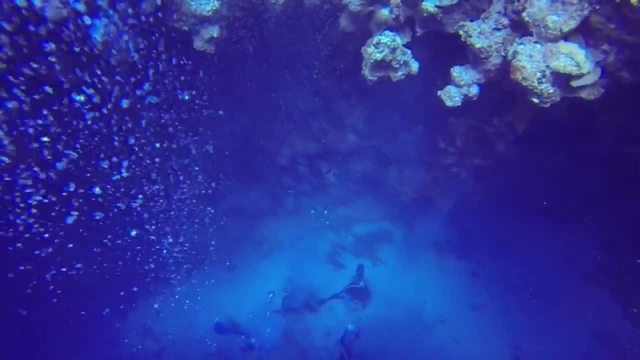 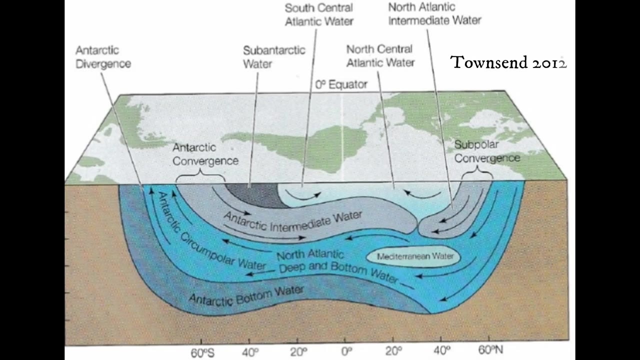 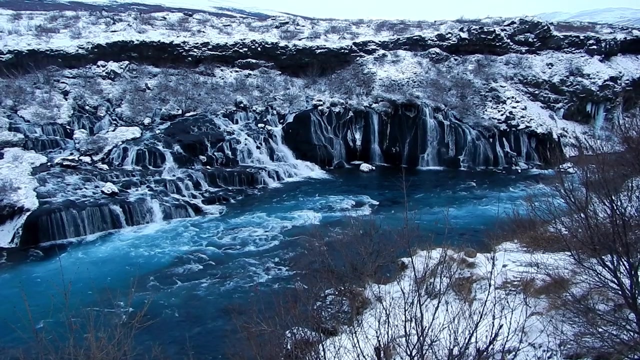 slide underneath a lighter one, and this vertical movement is called thermohaline circulation. These stratified water masses are given names. Near Antarctica, during its winter, the deepest and densest water on earth is created, known as the Antarctic bottom water. The cause is the 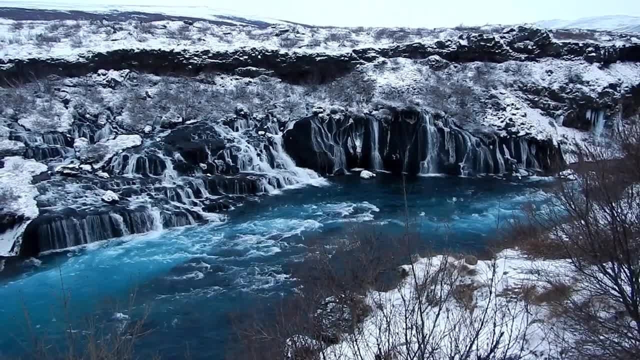 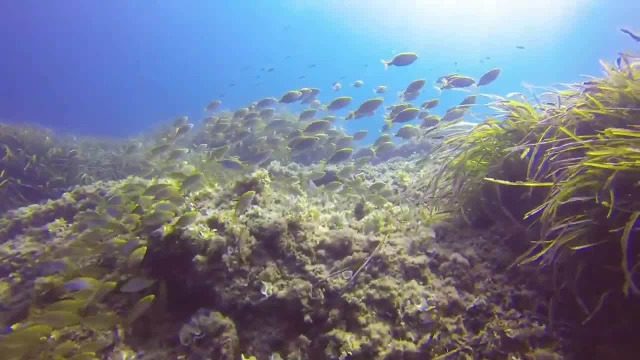 formation of ice, which makes the water very cold and saline. In the Mediterranean Sea, a water mass exists called the Mediterranean intermediate water. Although this remains warm, the high evaporation levels from the arid climate makes the water salty enough to sink to the bottom, where it can then. 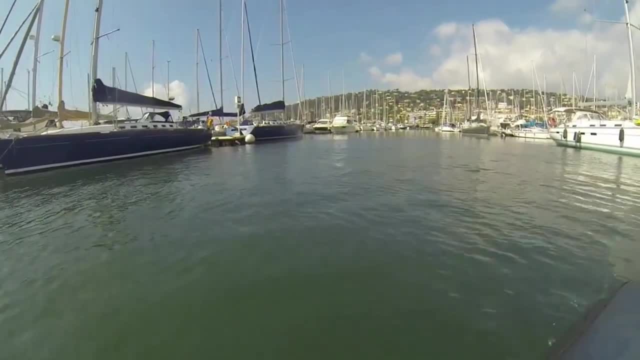 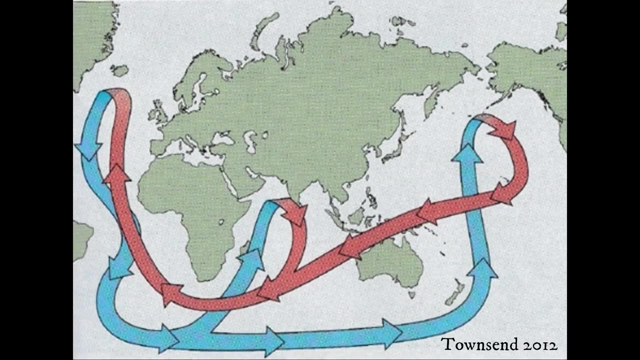 flow through the Strait of Gibraltar and drift in the middle of the ocean. The water that flows through the strait of Gibraltar and drift in the depths of the Atlantic. Because these slow, density driven currents provide a continuous mode of interconnected transport, the process is known as the 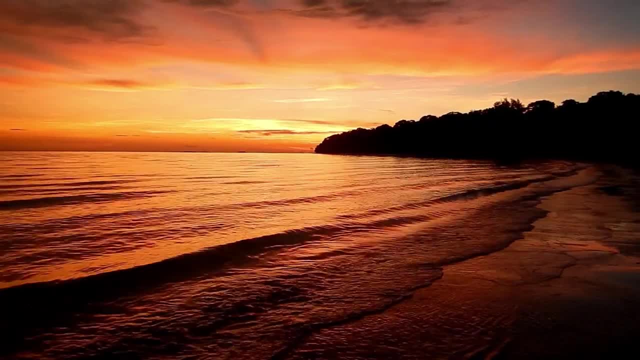 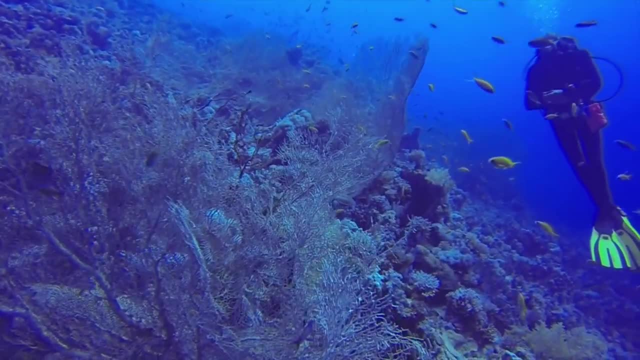 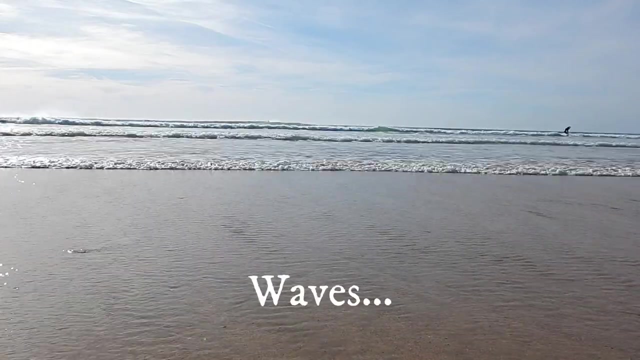 Great Ocean conveyor belt. It is a very important cycle which, in return, influences the planet's climate and atmospheric processes. Oxygen and nutrients are provided to hostile areas to support marine life. Wind is also the common cause for waves, which cause the sea surface to undulate. For waves to 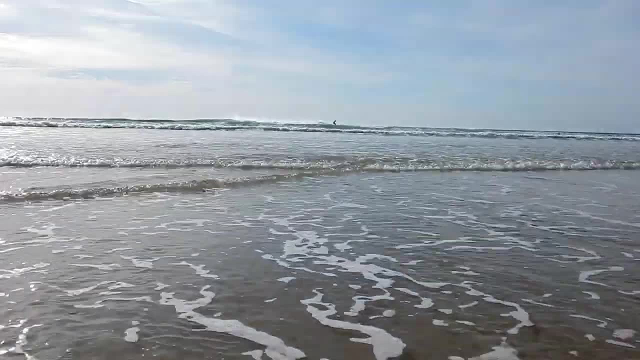 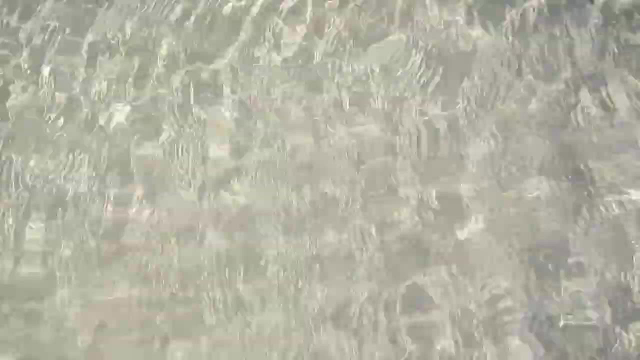 form, the wind will need to blow for a suitable duration and speed over a significant distance and area known as the fetch Ocean. surface waves are the result of a disturbing force such as wind, which are counteracted by a restoring force. Wind transfers its energy by lowering air. 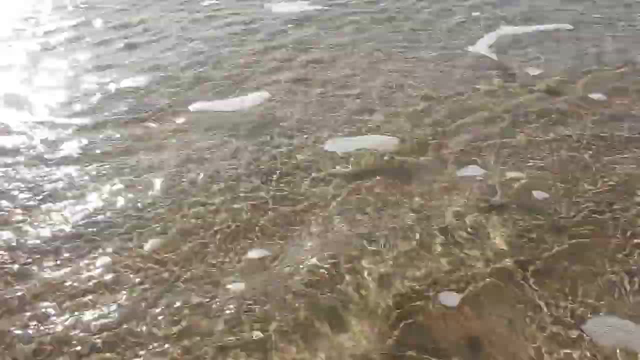 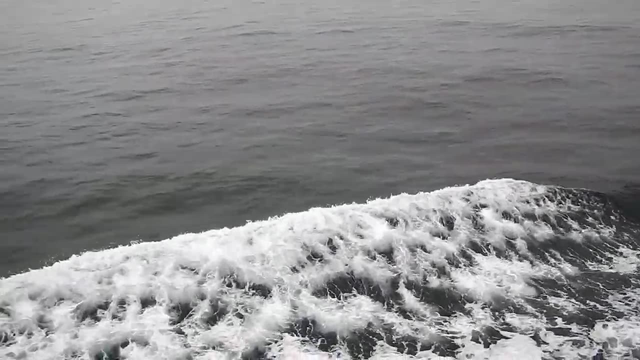 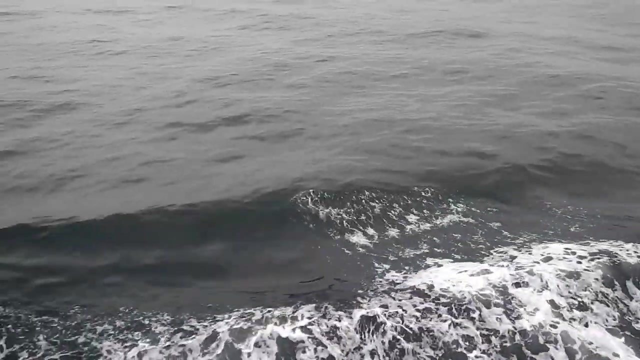 pressure which can lift water into ripples, Tiny capillary waves are created first, less than 1.73 centimeters in height. The biggest restoring force on petite capillary waves is surface tension from strong hydrogen bonds in the water. When the wind continues and the wavelength exceeds 1.73. 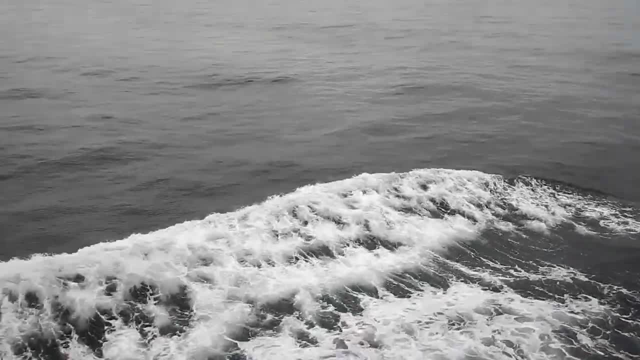 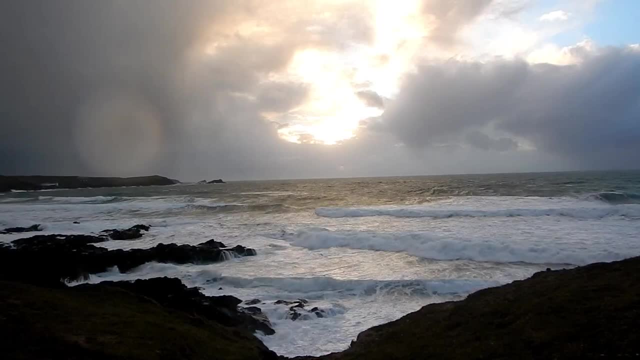 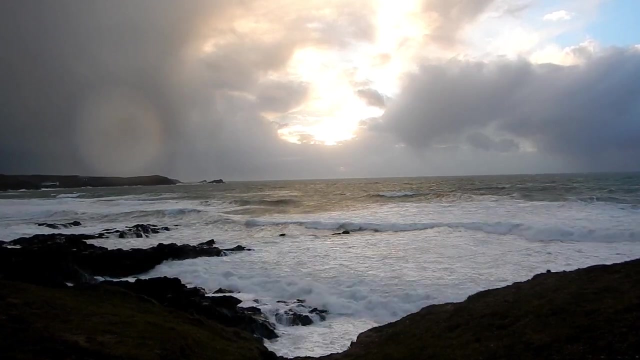 centimeters, gravity takes over as the dominant restoring force and a surface gravity wave has be formed. Because waves travel far across oceans, it could be assumed that the water particles are making the same long journey. However, in reality, it is only wave energy and form that travels The water. 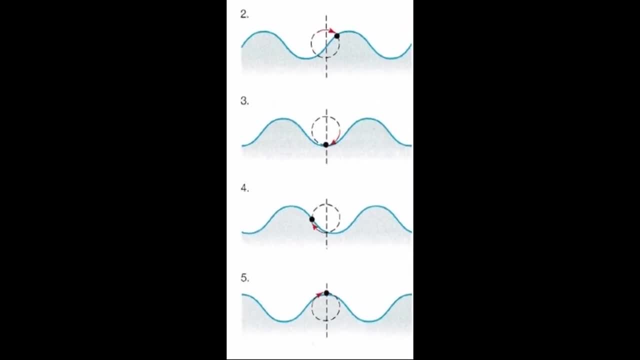 itself is scarcely moved and instead travels around and nearly perfect circles of wave orbit. These elliptical paths happen as, so any strange current moves around the waves. paths happen as surface water particles are caught up in passing crests and troughs. The diameter of the surface orbit will equal the height of the wave. 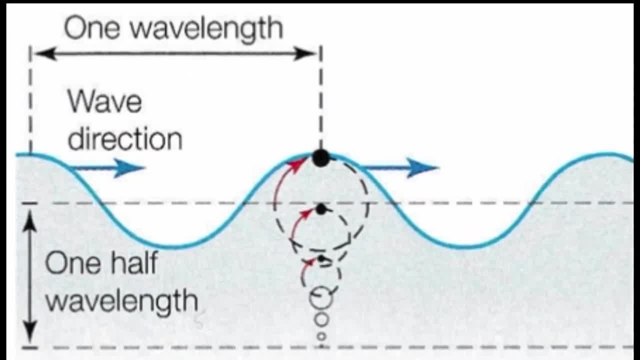 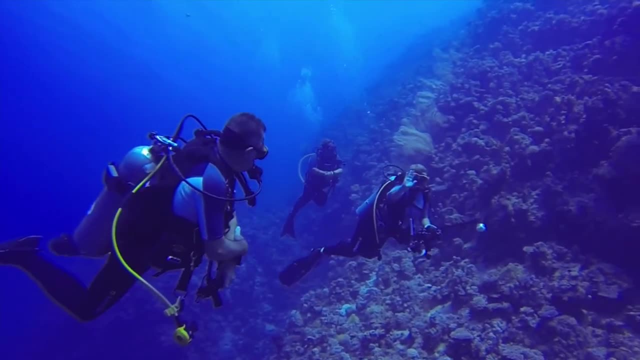 Water below the surface also travels in orbits, but their diameters decrease with increasing depth. Relatively quickly, the downward orbits will diminish completely at a depth one-half of the wavelength. Scuba divers may have experienced this phenomenon by starting their dive in rough swells and 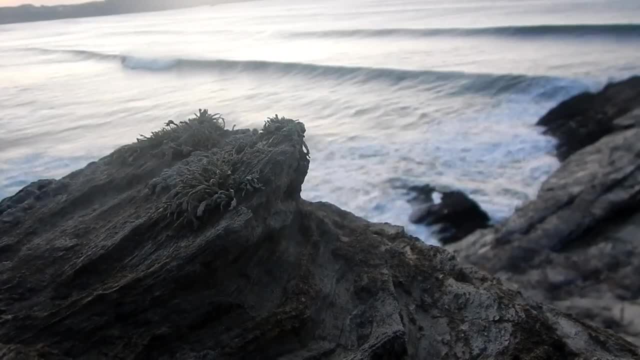 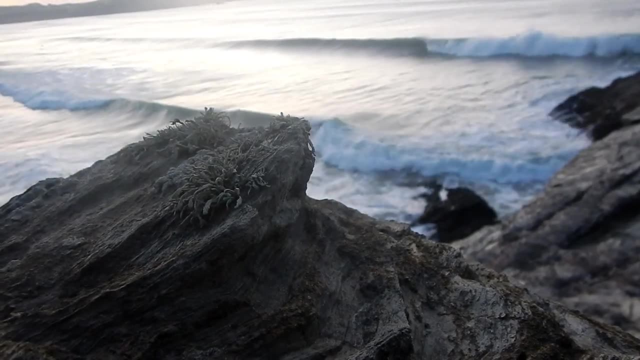 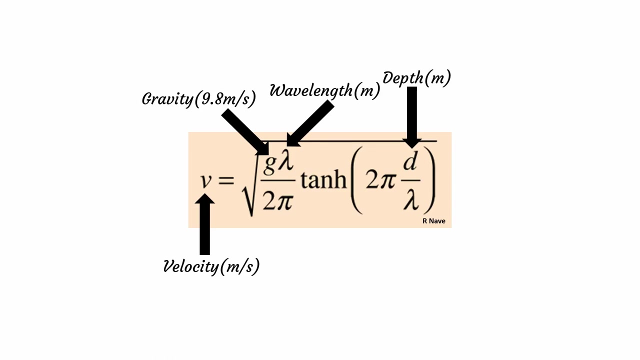 eventually descending into calm waters. If a gravity wave enters water depth shallow enough, the seabed will interfere with its wave orbits and the wave is slowed by friction. This equation can be used to determine the speed of any gravity wave because it encompasses the influence of both wavelength and water. 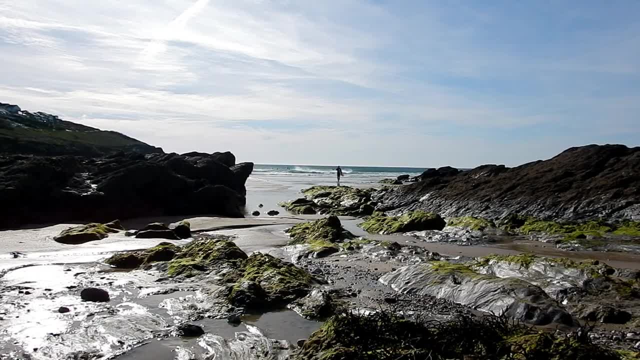 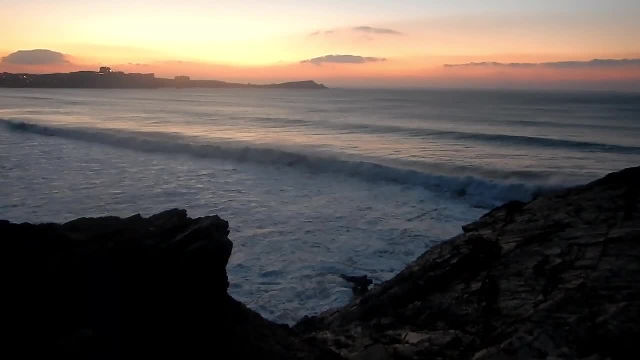 depth. When waves reach shallow waters, their steepness increases as the wavelength shortens. A critical steepness is met when the ratio of wave height to wavelength surpasses one to seven And the wave collapses on itself as a breaker. The steepness of the sea bottom. 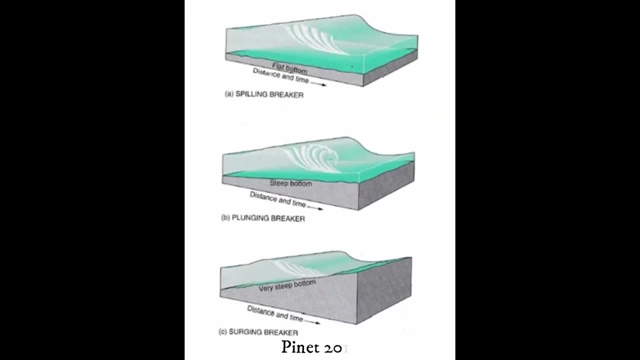 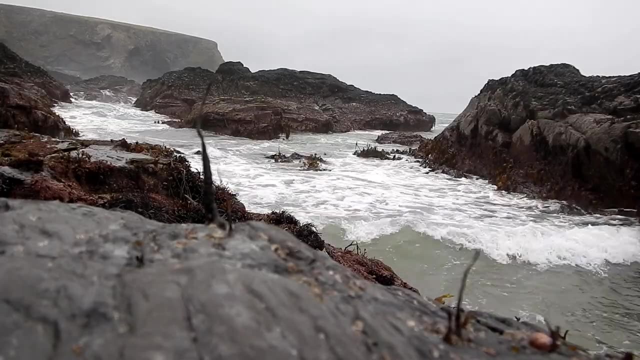 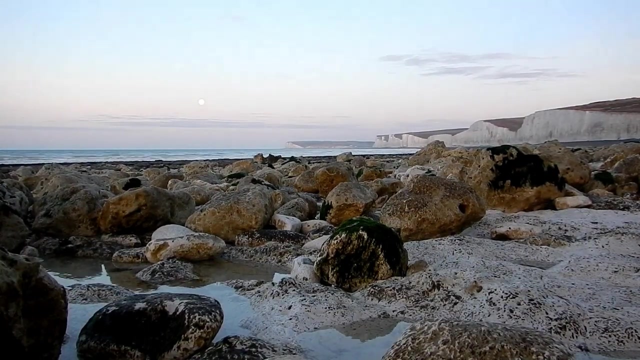 will determine if the breaker type is spilling, plunging or surging, due to the wave shape and how it releases its energy. Tides are the largest of ocean waves, although they are not commanded by winds but by gravity. The gravitational pull from the moon and the centrifugal force in the opposite direction causes the. 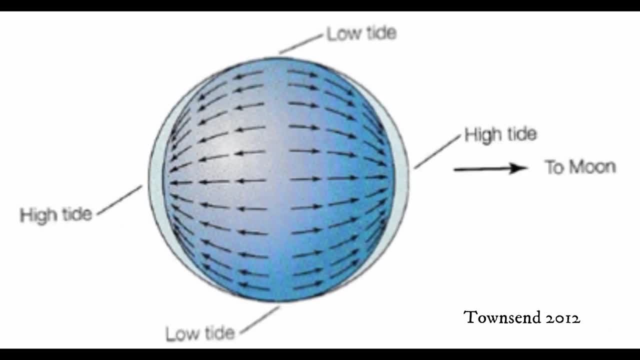 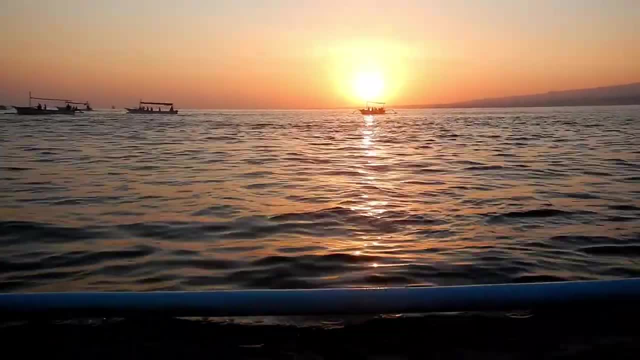 oceans to bulge either side of the earth. These are the high tides which the earth rotates through. However, it is the Sun which amplifies this gravitational pull. Larger spring tides are created when the Sun, Earth and Moon are in alignment, during new or full. 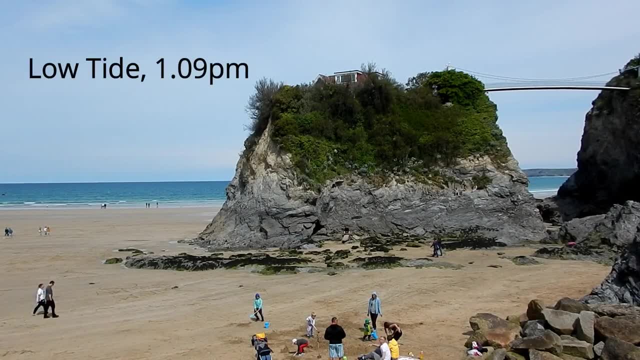 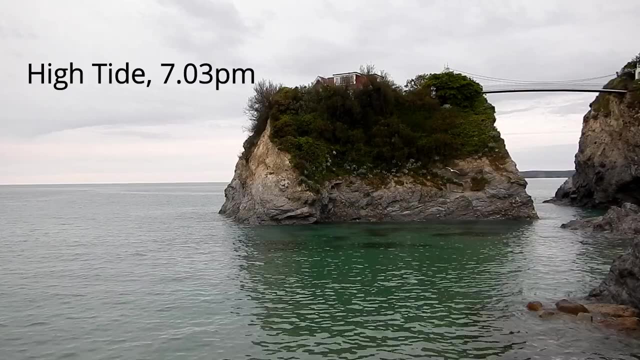 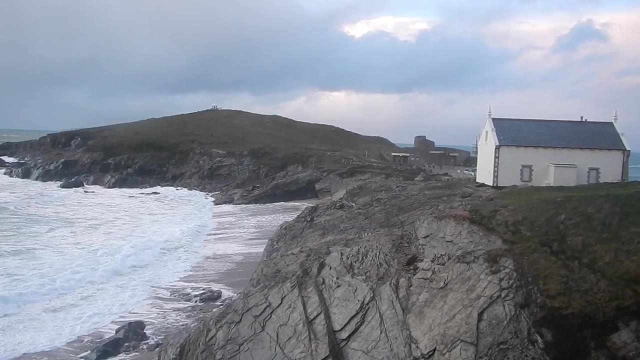 moons. So far, these theories have followed a simplified model of the tides known as the equilibrium theory, which assumes that the earth has no landmass and that all water is a constant depth. Water is considered to be static and in equilibrium with the tide raising forces. The dynamic theory of the tides is a